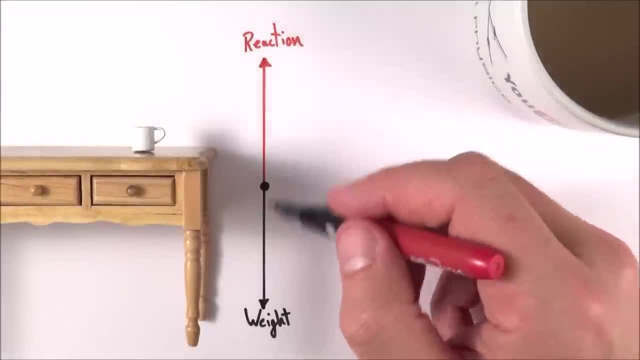 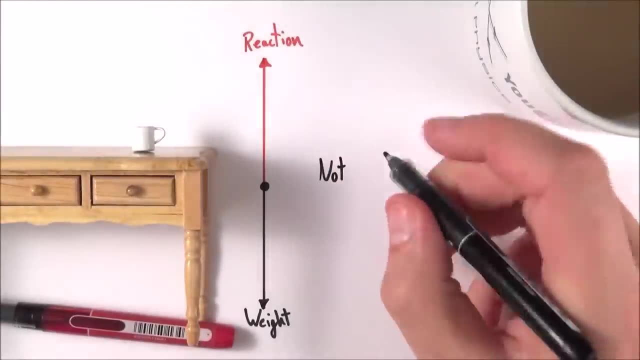 what people think is okay we've got. maybe the reaction force is equal and opposite to the weight and therefore that's an example of Newton's third law, But this is not Newton's third law. The reason that this isn't Newton's third law is that what we have here are different. 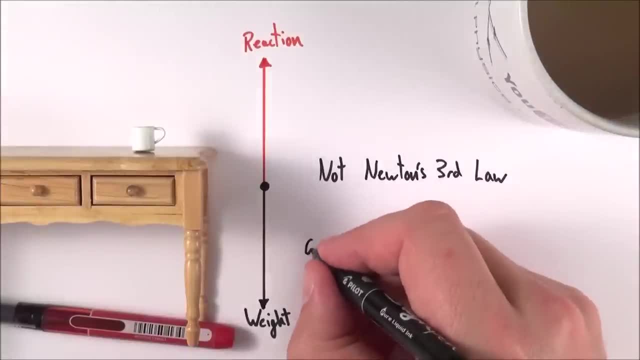 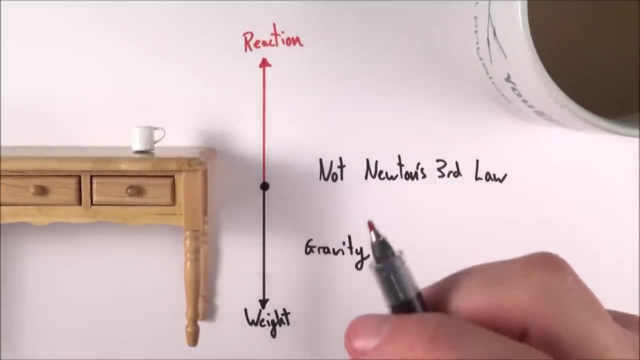 types of forces. First of all, the weight force is provided by the gravitational attraction, So this force is a. The reaction force, though, is due to the interaction between, effectively, the electrons in the bottom layer of this cup and the electrons in the top layer of the table, And this is 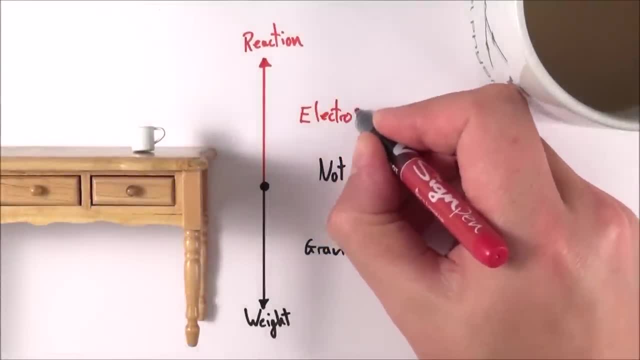 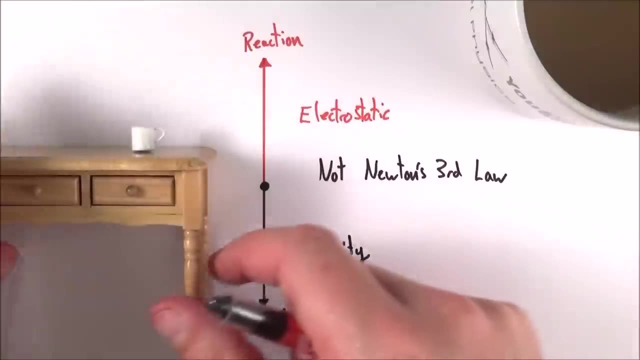 where we have this kind of electrostatic repulsion. So what we have are two different types of forces. They might be maybe an equal size, perhaps if we ignore the fact that this is on the Earth and it's going round and round. But what we need to really look at is the 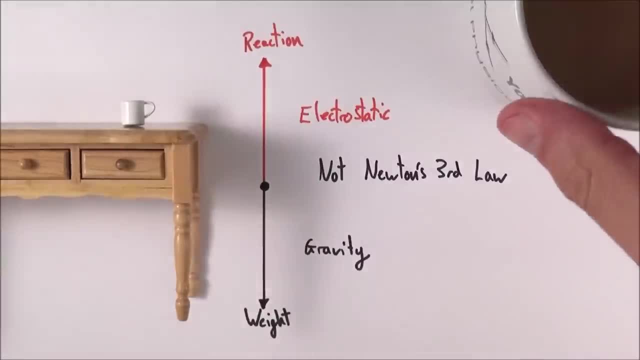 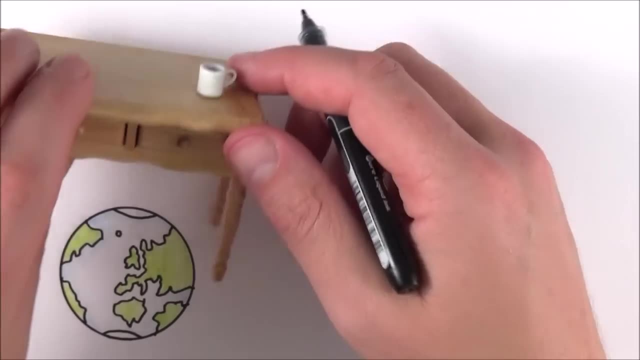 pair of forces that are actually involved. So, first of all, I'd like to think about the downwards force, perhaps, of this mug, which is acting downwards, And if we maybe just ignore the table for the moment, this mug is experiencing a force downwards that we call weight. 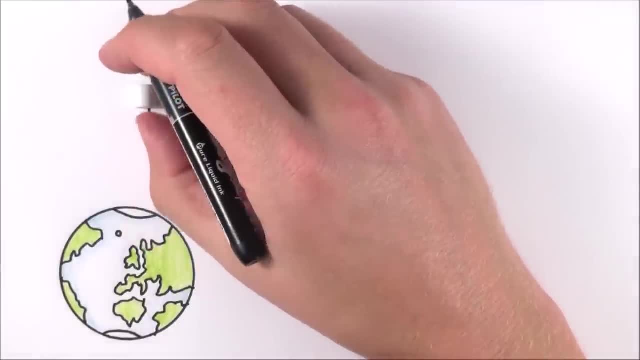 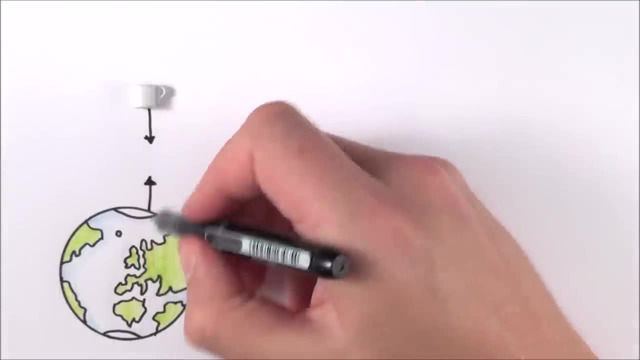 And so I'm just going to put this down here a bit like that. and the reason it experiences weight is due to the gravitational attraction, but the Earth experiences an equal and opposite gravitational attraction upwards up towards the mug, And in actual fact, this force here 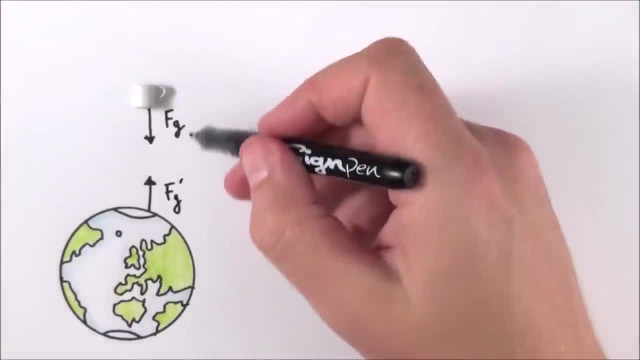 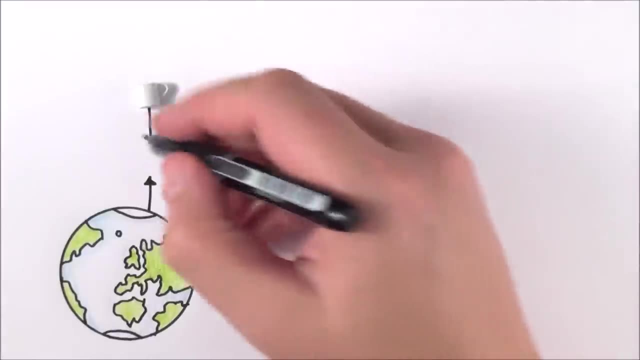 Fg and this one. here Fg, they're exactly the same size, And so this is an example of Newton's third law: Here's object A and here's object B, So here's A and there's B. 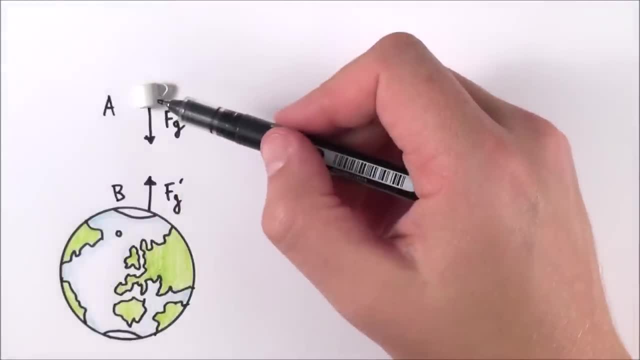 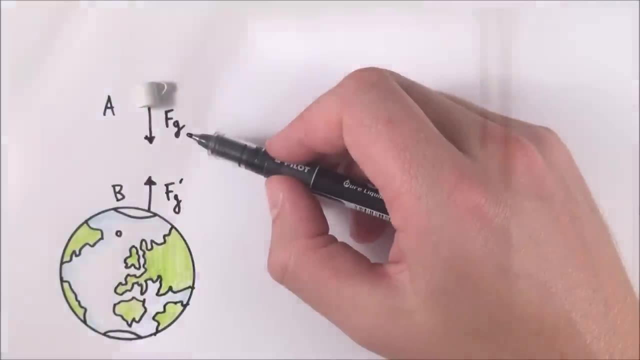 And therefore Newton's third law still applies. The force of the mug on the earth is equal to the force of the earth on the mug, and they are equal and opposite in size and they're of the same type. Now the other force is effectively the reaction force between the mug and the table. 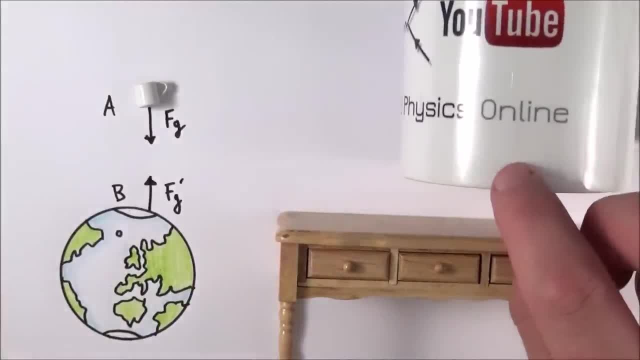 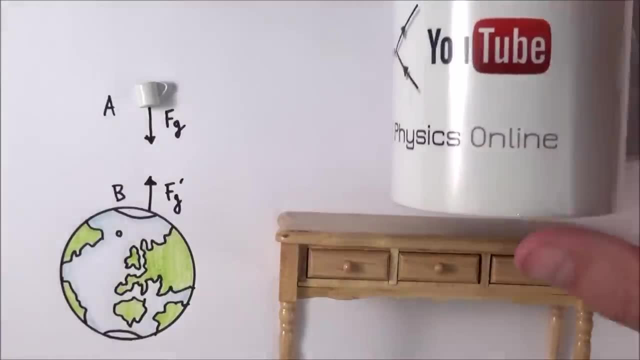 And the reason for this is that in the bottom layer of the mug there are all these electrons which are basically the outer electrons around all the atoms. And these electrons, when they get closer to the table, they're going to start to get closer to the electrons in the top of the table.